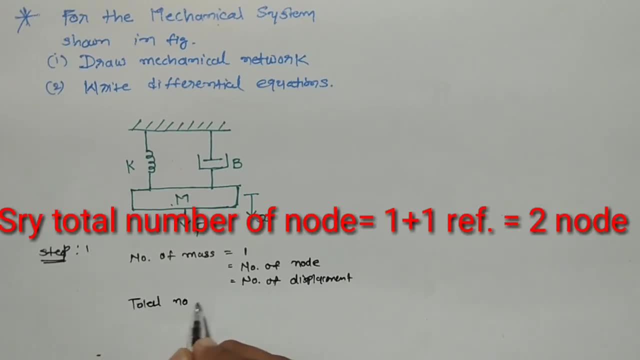 Now total number of mass is equal to one node plus one reference node, So that there are two nodes with including reference node. So total number of node is two. So I am drawing here mechanical network. First of all I am considering node X, because one node and one is reference node, So that I am writing here, drawing here. 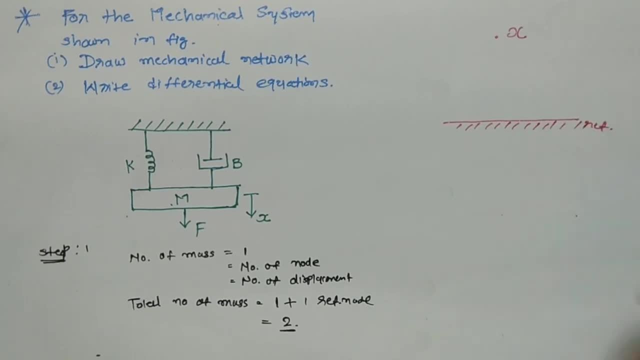 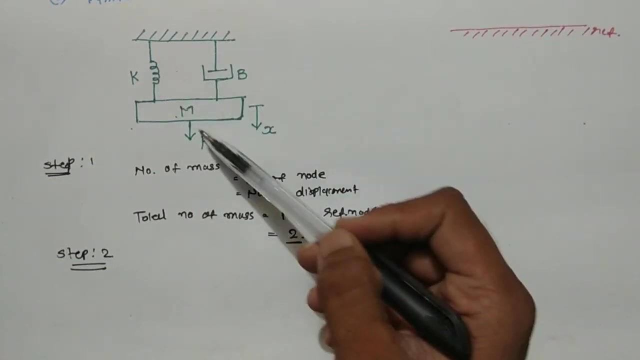 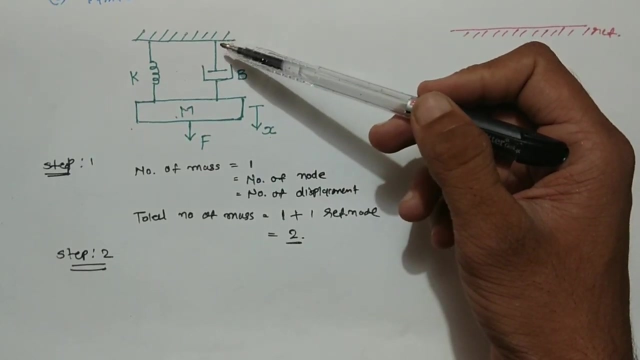 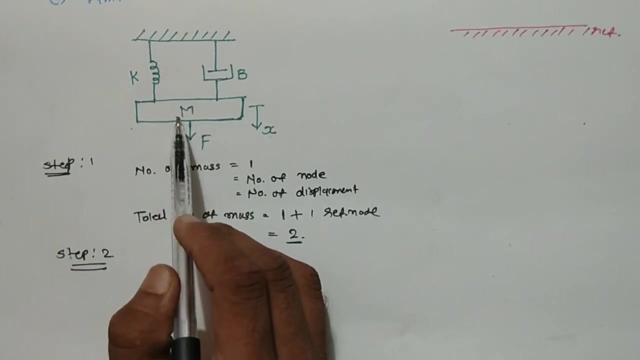 Second one is reference node. Now step number two. In step number two, all element connected with node to reference. So first of all, one most important thing is: whatever mass is given in mechanical network, it is always connected with node to reference Means. whatever mass is there, it is connected between node to reference. 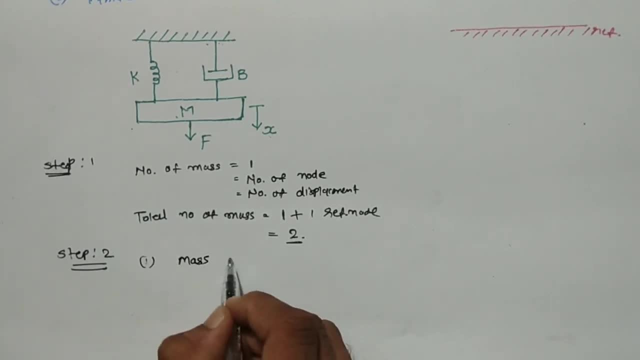 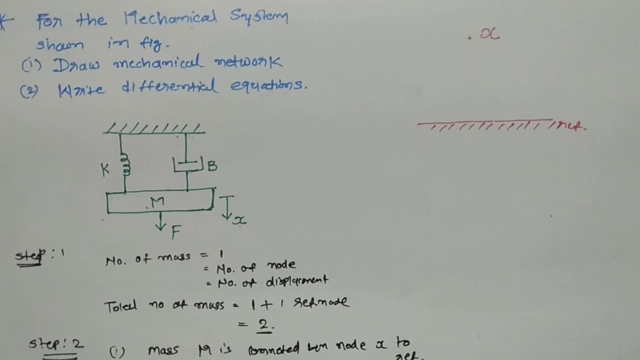 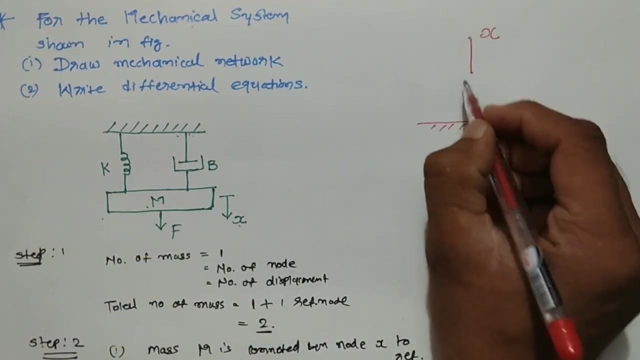 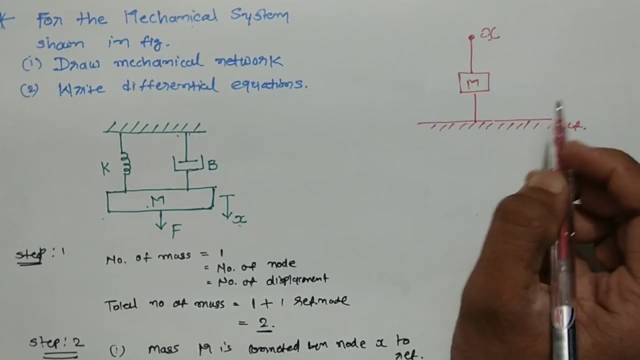 So that first of all mass M is connected between node X to reference, So that I am connecting here mass M in between node to reference, So that first of all that is mass and is connected between node X to reference. Whatever mass is there, whatever mass is there, it has to be connected between node to reference. 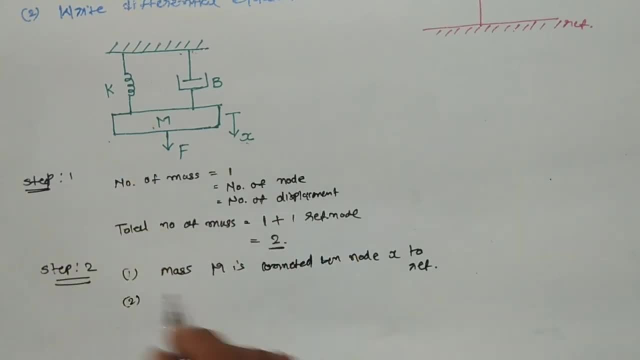 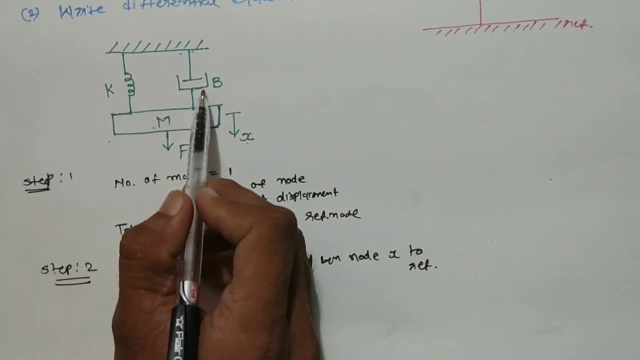 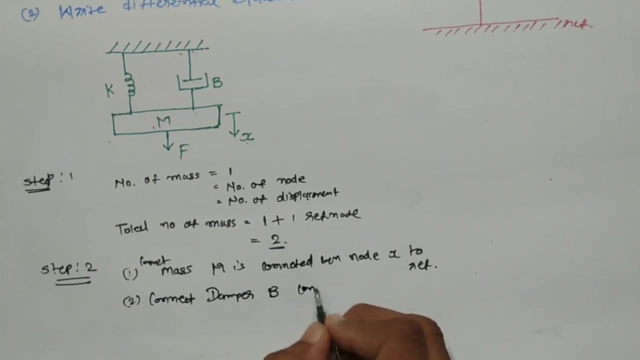 Now connect, connect damper B, damper B between that damper B is connected with mass, So that is connected between node to reference, So that damper B is connected between node X to reference. So that I am connecting here, So that I am connecting here. 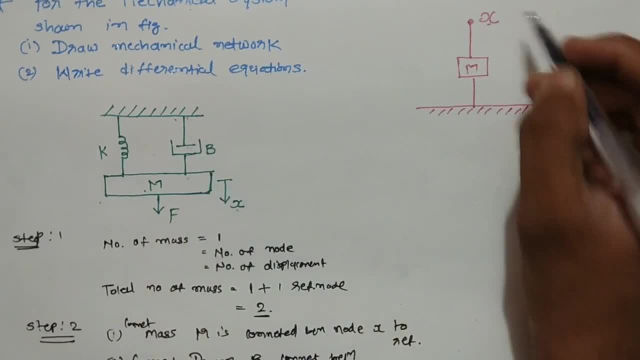 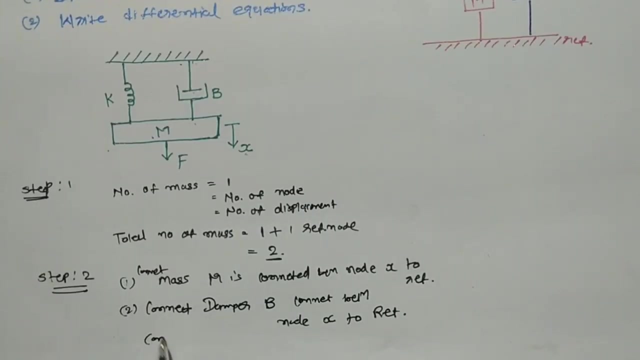 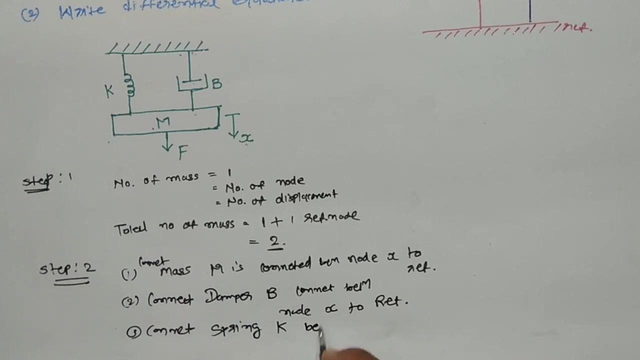 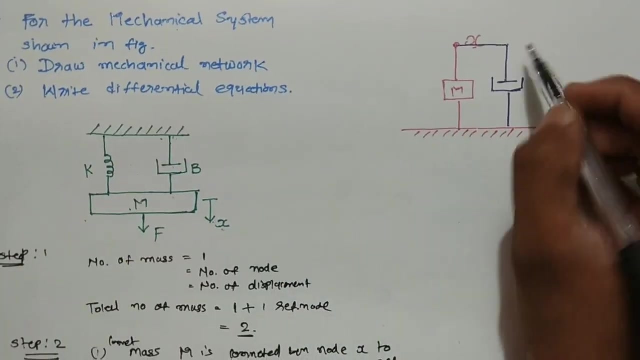 Damper B in between node to reference, So that that is node and here one is. damper Is connected between node to reference. Now connecting, connect spring K between node to reference, node X to reference. Here spring is connected between node to reference. 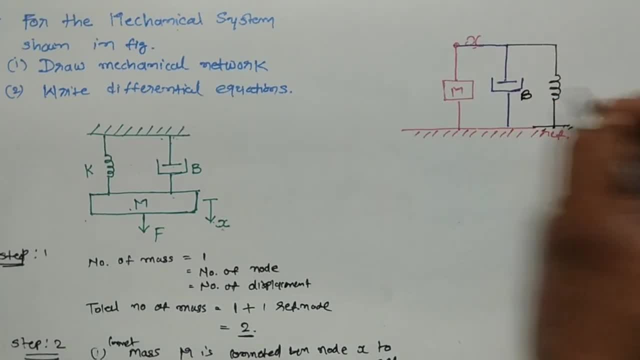 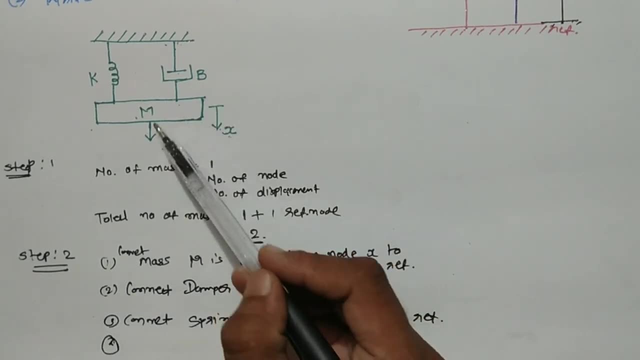 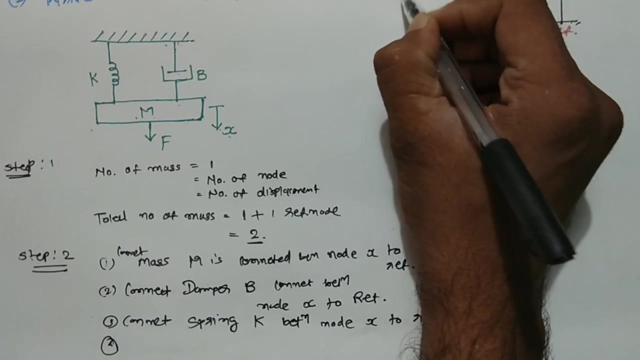 That is reference node, That is damper and that is spring. Now force is applied to only mass, So that there is some displacement, So that force is going towards to node X, So that I am applying force here, F, towards to. I am applying force here. 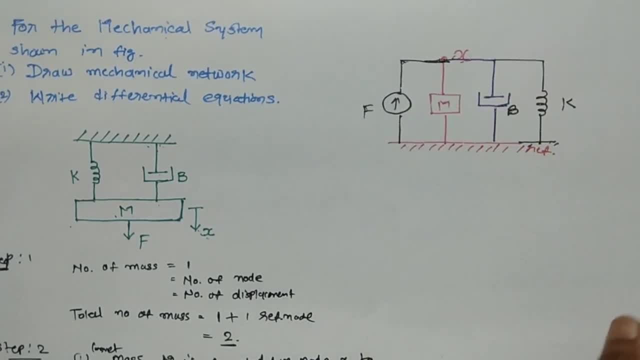 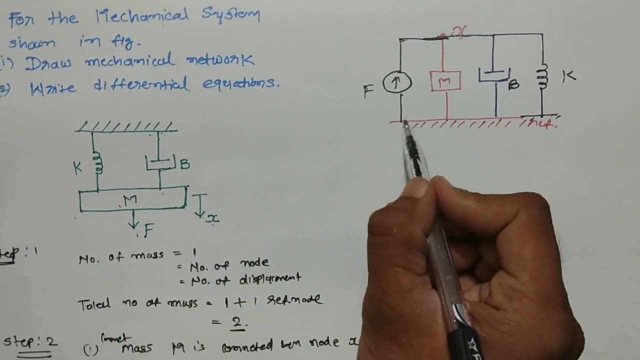 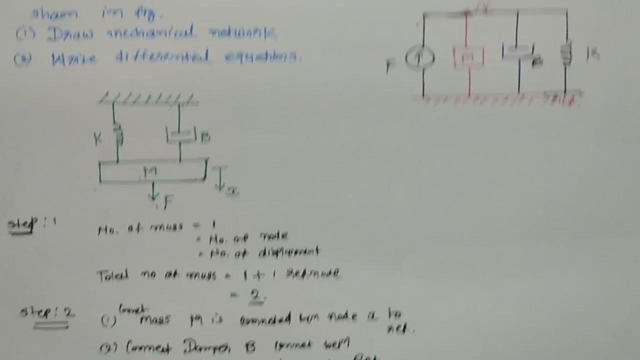 towards to node X, Because here the force applied to the top of the mass, So that force is directed towards node, So that I am applying force towards node. That is your step number 2.. And then, after drawing mechanical network, Now step number 3.. 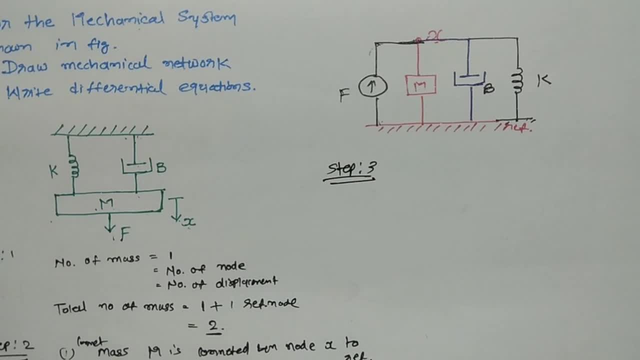 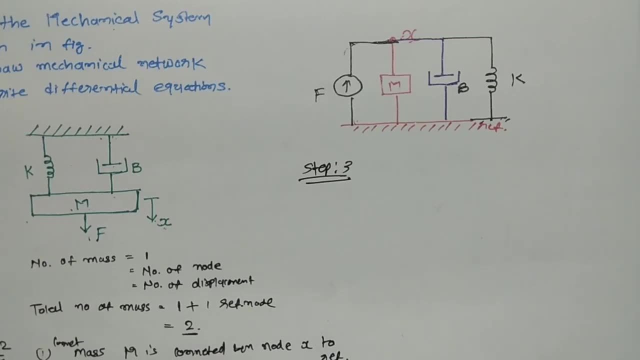 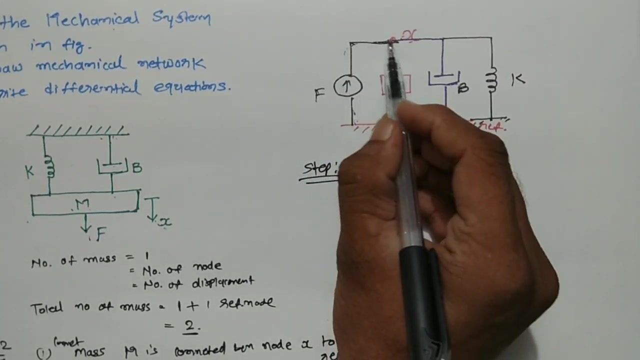 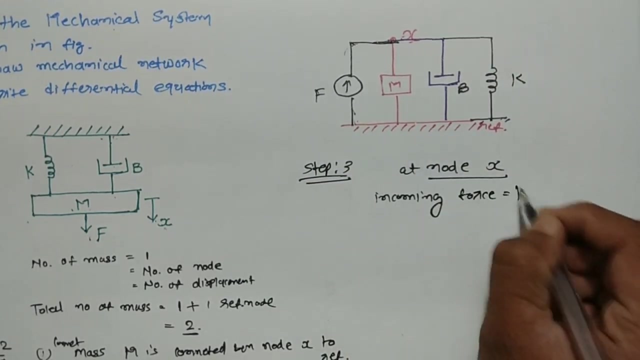 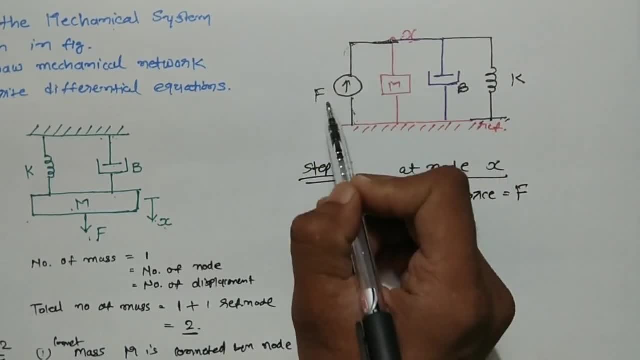 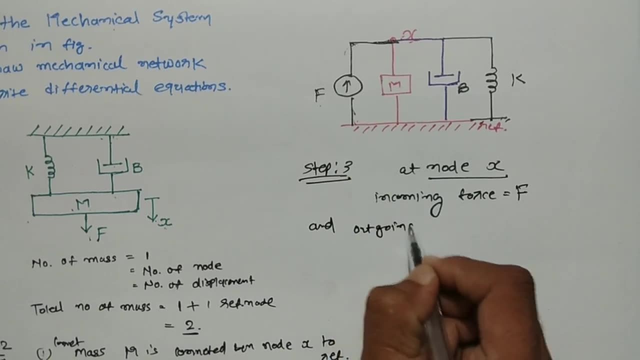 Here towards node X, which is applied force F and outgoing force. outgoing force are happen on three element: Mass, damper and spring, And that is given by. force apply on mass is given by mass into acceleration Plus force apply on damper, that is given by